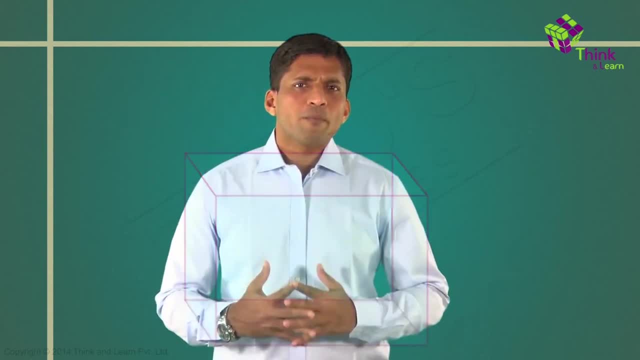 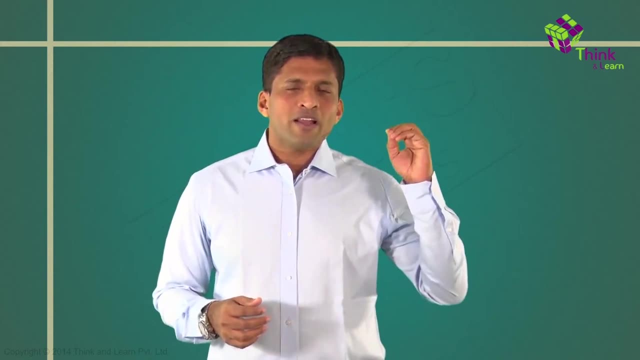 I will get solids which are three dimensional. Now let's simplify geometry using common language And in simple language. let's try interpreting one to many. So if I try interpreting one to many, I will get one to many. So if I try interpreting one to many, I will get one to. 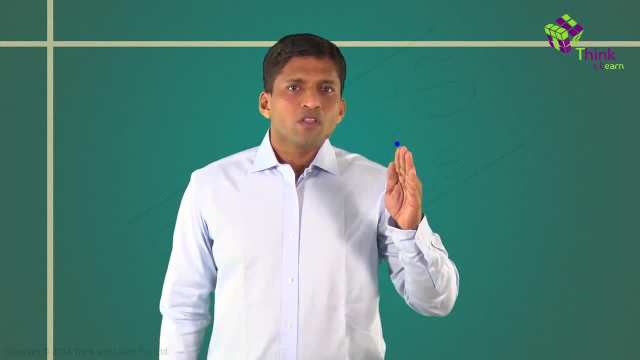 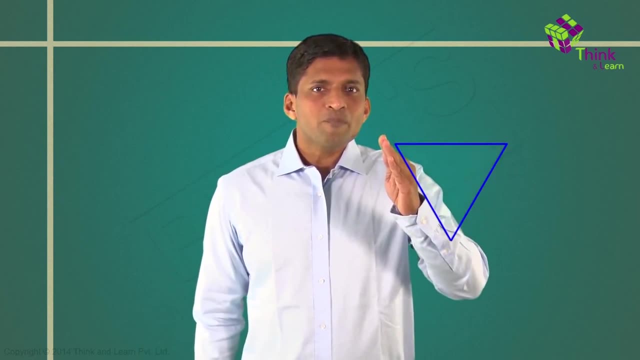 many in a diagram. I start with a point. Lot of them together, I get a line. Two lines to get an angle. Three lines, I get a triangle. Make this one to many, So two triangles together I get a quadrilateral. Keep on adding triangles. I will get trapezius and pentagons and hexagons. And if I do, 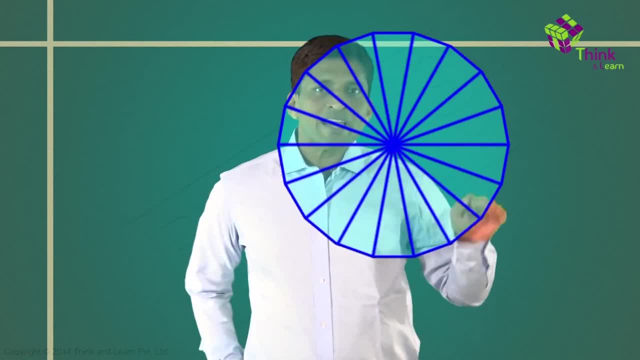 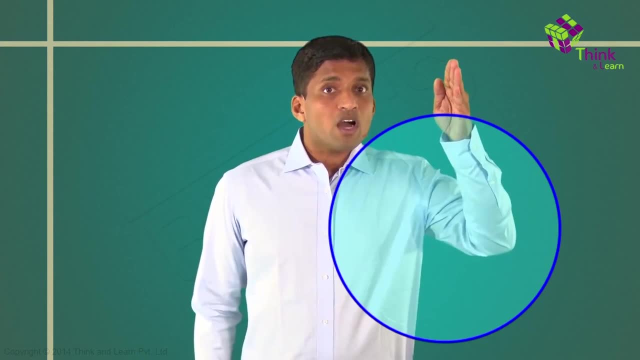 this many more times. infinite number of triangles. I get a circle like this, So circle is nothing but one. to many Now cut the circle, straighten this out. I get a line, and that's where we started from, So line can. 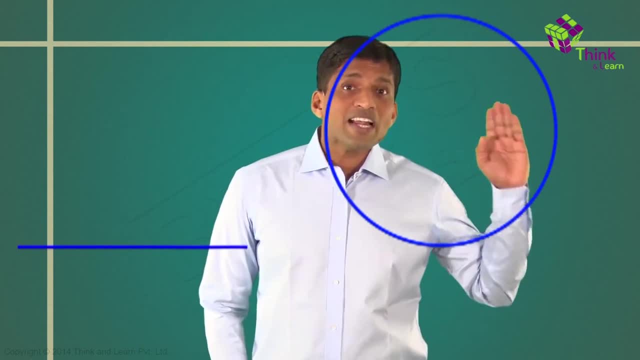 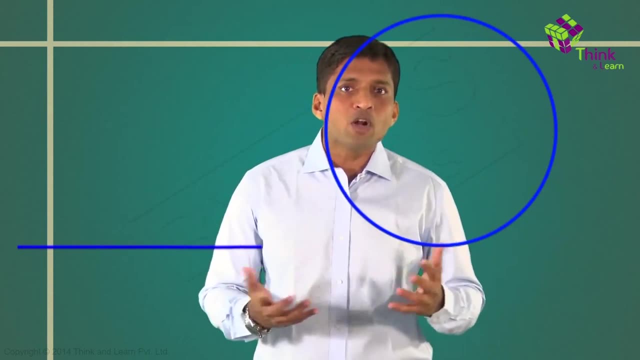 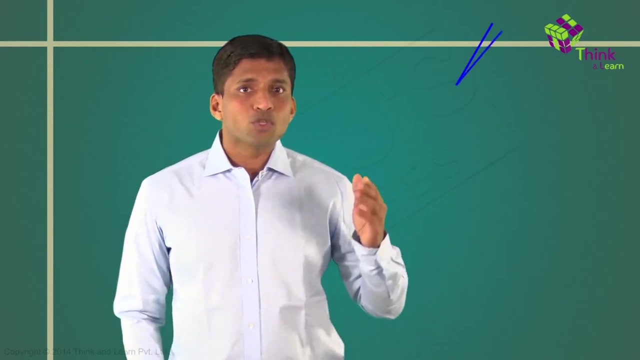 be taken as a circle with infinite radius. Circle can be taken as a polygon with infinite lines. Line to a circle and everything in between is what we need to learn in geometry, in plane geometry. So it's very simple. So we'll first start with two lines together. We call them angles. Next chapter: 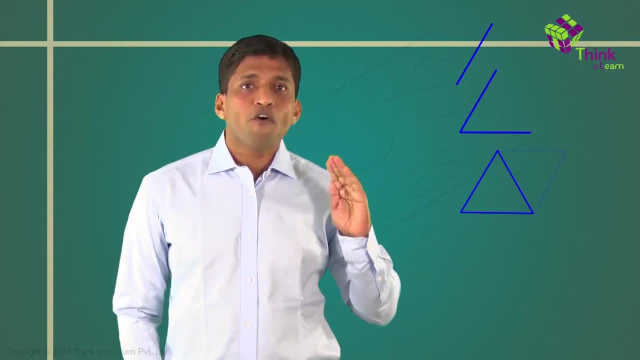 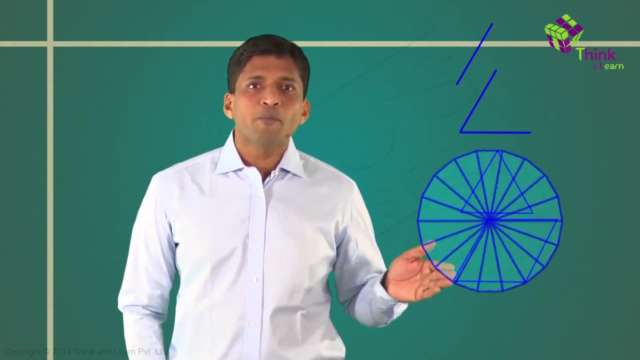 will be three lines together, So we'll start with two lines together. We call them angles. Next chapter will be three lines together. Triangles, Four of them together, We learn next. We call them quadrilaterals And the next chapter will be infinite number of them put together. We call them circles, And it sounds very. 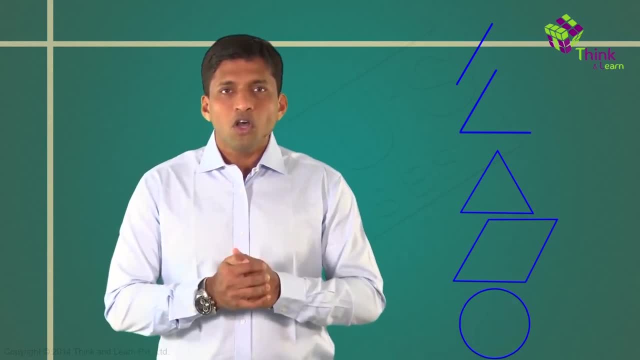 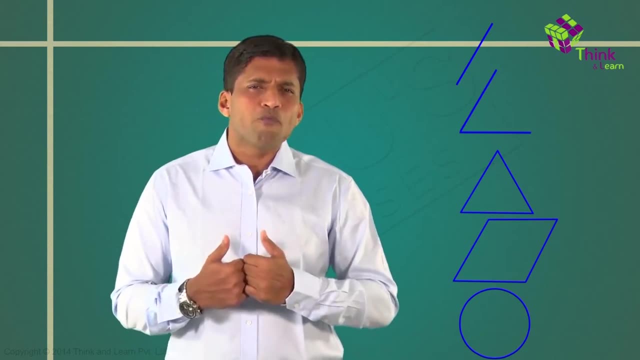 simple right. It's actually much easier than what you think. So geometry is going to be- it's anyway easy- and it's going to get much more interesting And you're going to find it. it's gonna become well below anyone's level very soon. 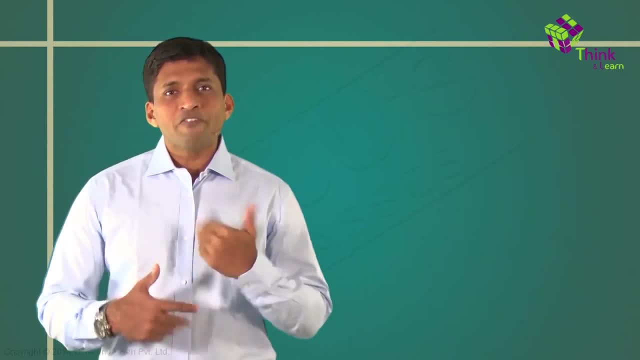 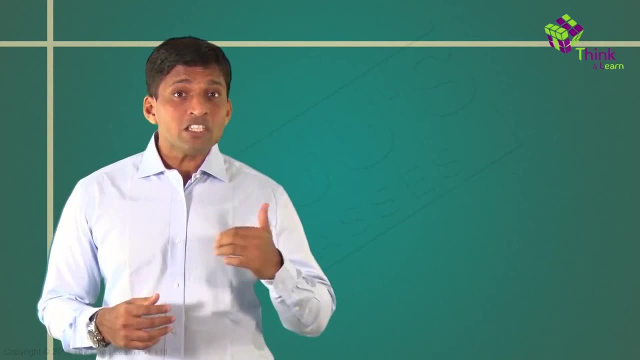 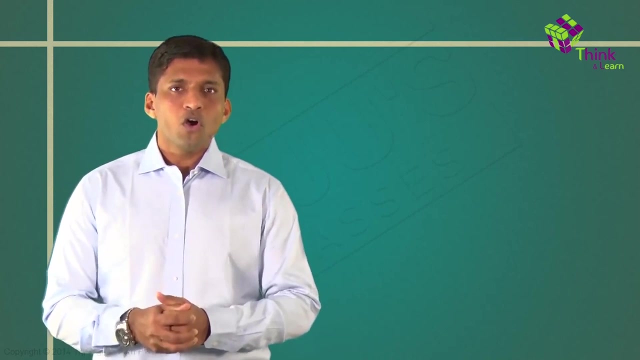 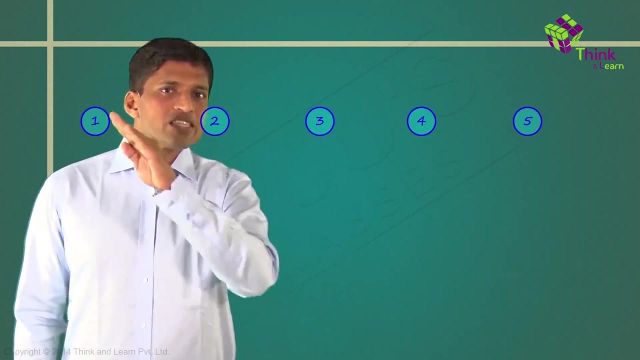 Now Let's understand geometry in a different way, but obviously in an easier way itself. So geometry can also be taken as number patterns visualized in diagrams. So let me help you understand why geometry is number patterns visualized. So if I start with the basic number pattern, which is 1,, 2,, 3,, 4, 5,, these are natural.